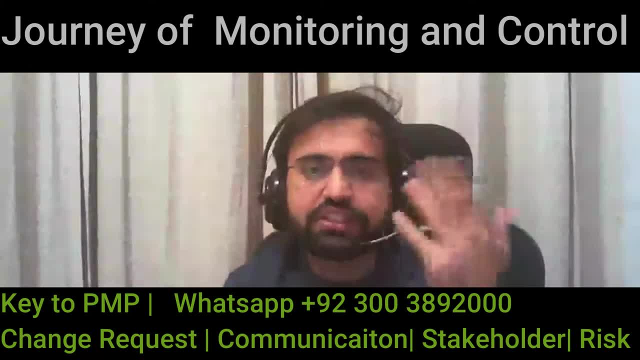 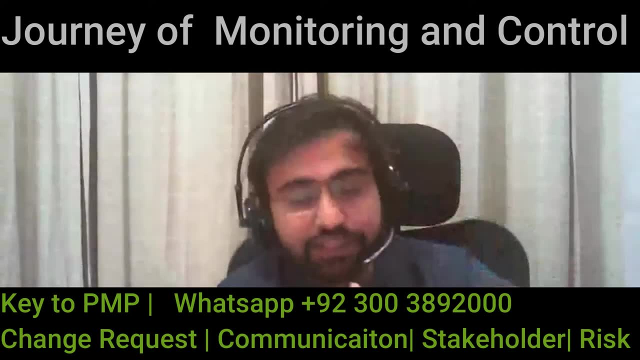 Further, we analyze in this process what are the reasons for this variance. We do cost-benefit analysis, we do root cause analysis to go to the real reason why the variance is there. Then we, from the alternate analysis, we see what are the options to follow and which is the number 1 or second. Then we, from the alternate analysis, we see what are options to follow and which is the non-reliable which is selected here. And then did that interview with, And then did that interview with this scenario with, to experience how this variances work as we готов. 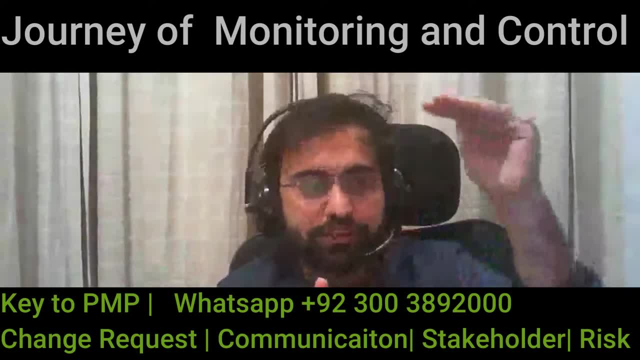 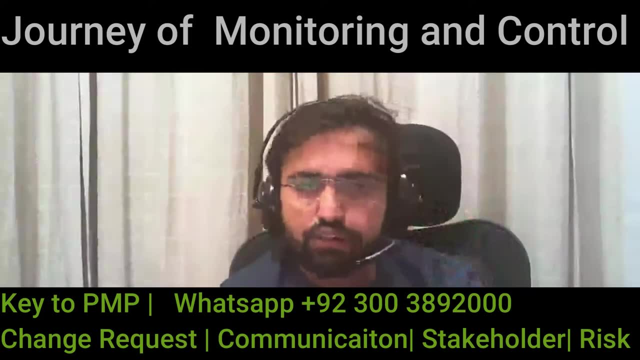 column, from the column, from the column, from opportunity for evaluation. I on video window. you have data only, we have follow and which is the number one option, and we combine cost benefit analysis with it. then we do basically control charts, all those control things. so variance is the first thing. this 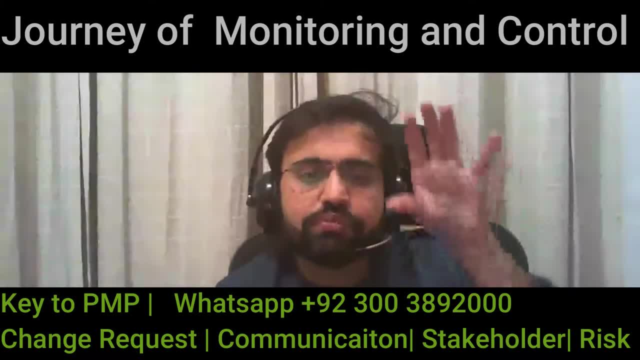 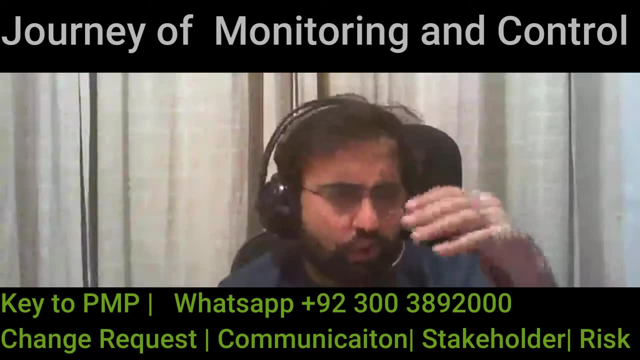 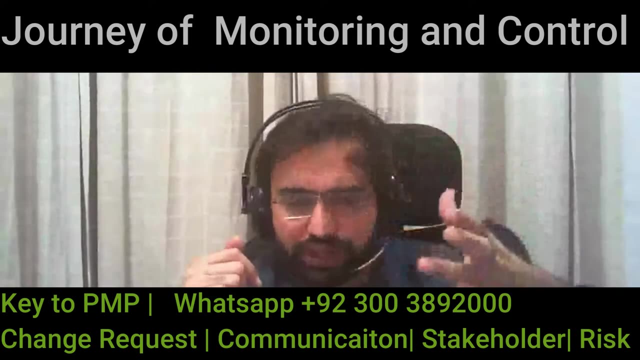 basically what is meant by variance. we are using project performance measurement, we are checking the performance of the project through appropriate tools, of course, and we qualify to quantify them through these things, and we recommend corrective actions once there is a variance that we have identified. the variance is negative, then we issue change request from validated scope. 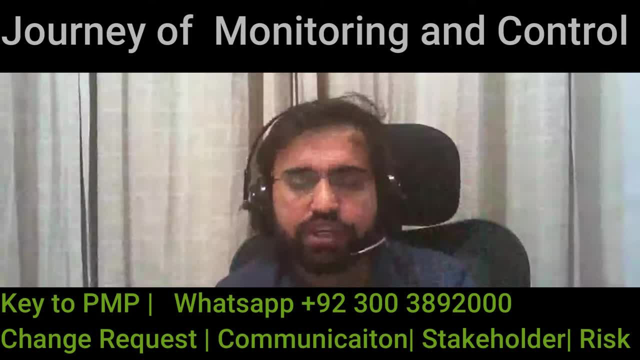 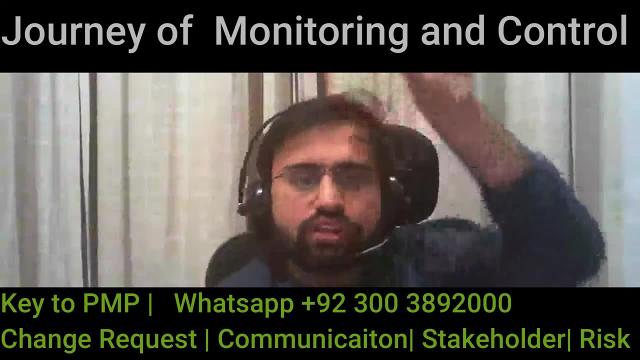 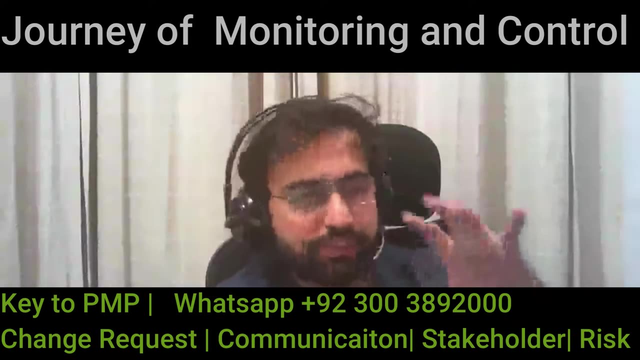 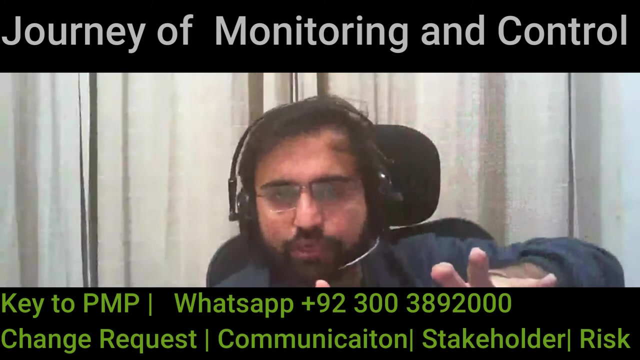 till stakeholders. all process, all monitoring and control process. generate change request. also monitoring and control project. also generate change request and all these change requests goes to one process. perform integrated change control. the first step is to see the variance- is a major performance. second step is to generate change request and approve change request. 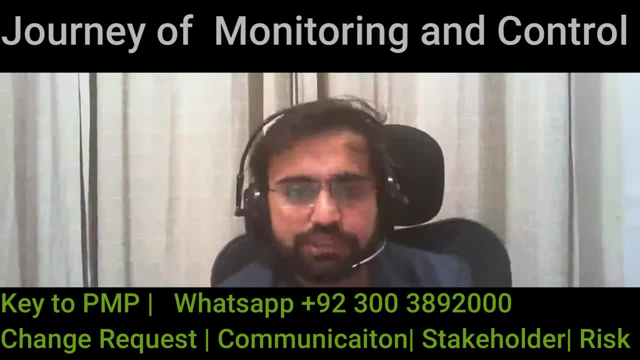 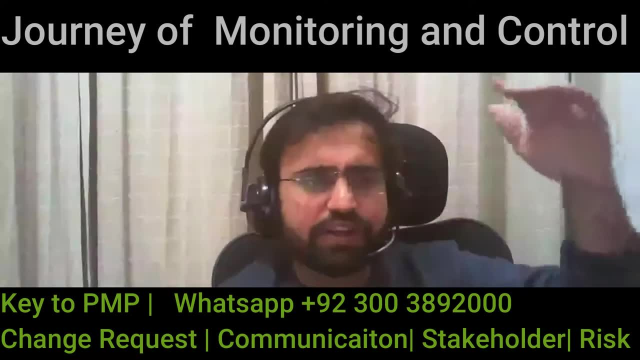 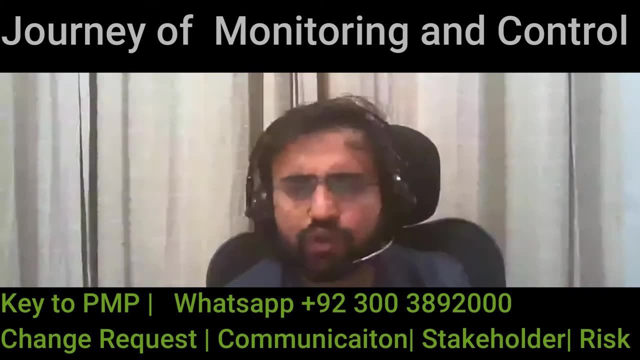 integrated through integrated procedure. and the third step is to check the deliverables. first we check deliverables internally in the control quality. we are verifying that we have met the agreed quality standards, using appropriate tools and technique, of course, to meet the business requirement. and then we get the formal acceptance of these deliverable invalidate. scope from that. 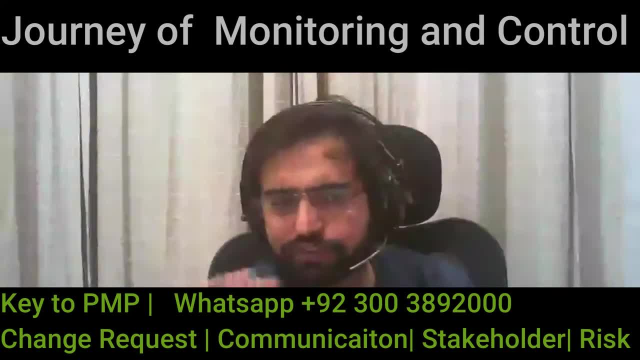 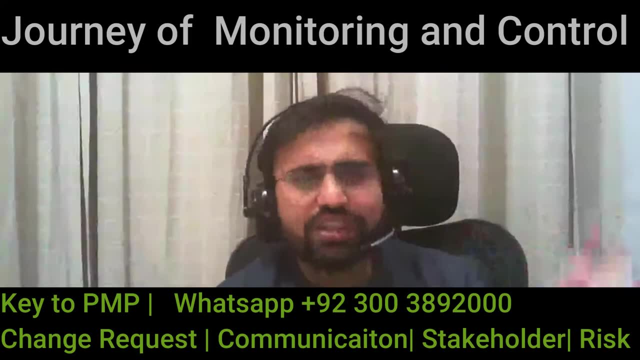 line we get the formal acceptance of deliverables from the client. of course, once you are producing deliverables you have to monitor the risk. you have to ensure no other risk gets there. you do risk audit to check the performance of the risk. you monitor and reassess the risk. 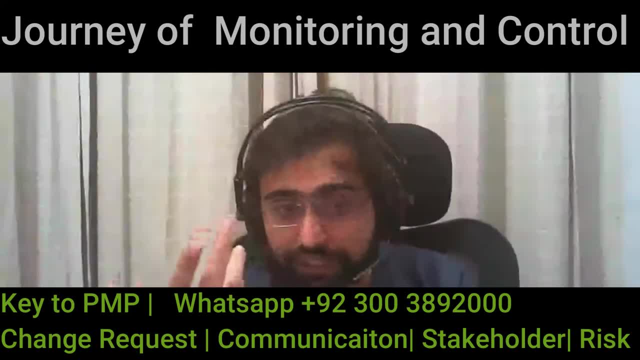 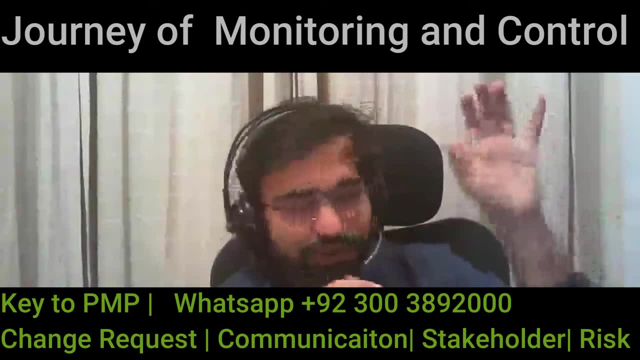 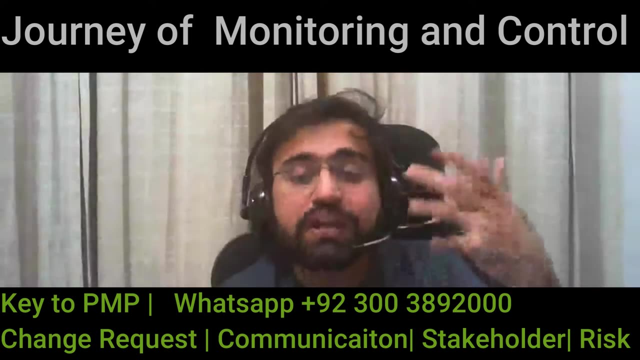 you check a residual risk. you basically check the secondary risk. all these things are there. now, once the risk has acted, it becomes issue. risk is probability into impact. the probability is 100, then it's an issue. we need to review the issue log, we need to manage the issue log. we need to update and, if they are, recovered, if it is necessary. 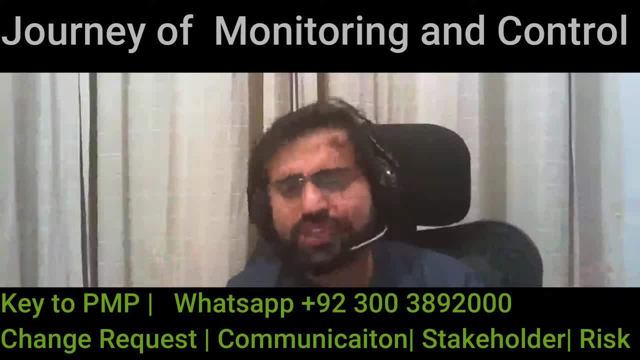 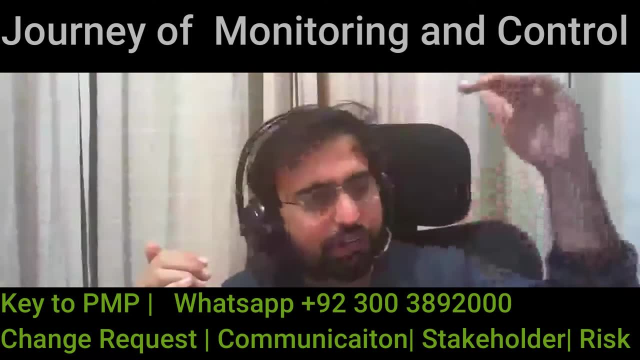 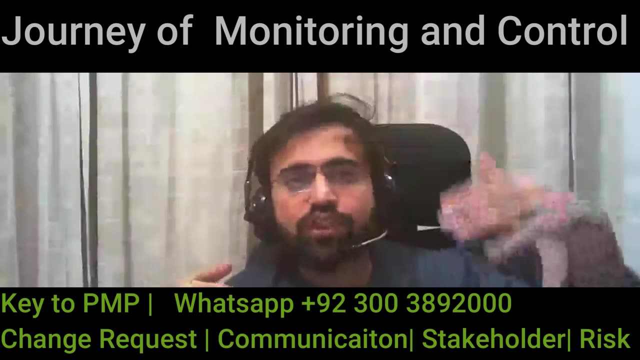 to determine corrective action by using, of course, tools and technique that are required for the issue. and then, in all the areas, whatever the risk has occurred, what are the variants have occurred and we have found out the reason, the variance. we write less and less. we document the lesson lines so that we can use that in future. 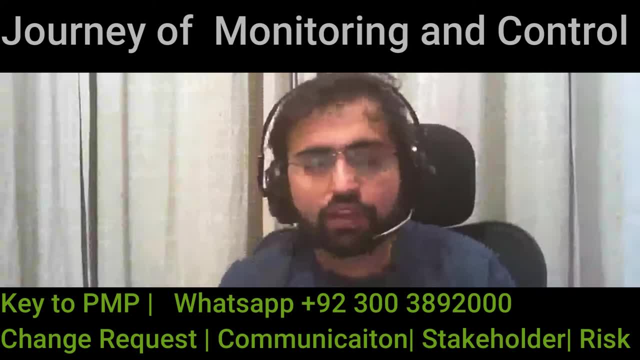 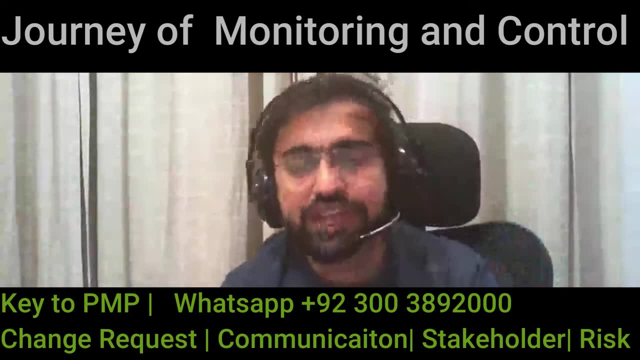 and of course, we, if we have done procurement, we close the procurement. here very important: in closing the procurement, we are inspecting the deliverables and if contract allows us, we are doing the audit of procurement process. and finally, if we do not reach to agreement, we have alternate. 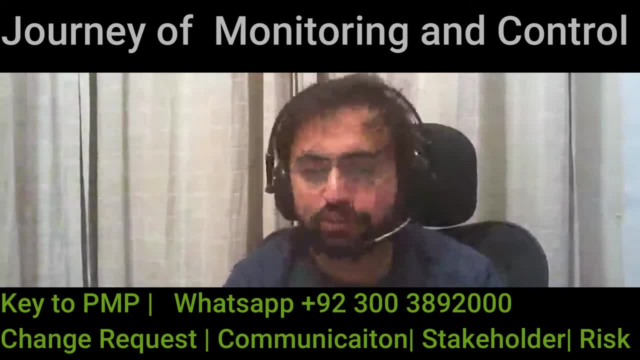 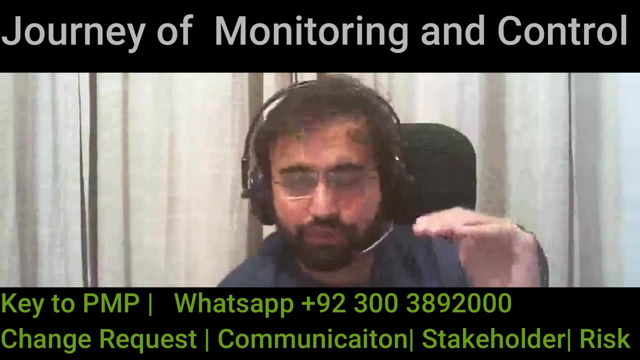 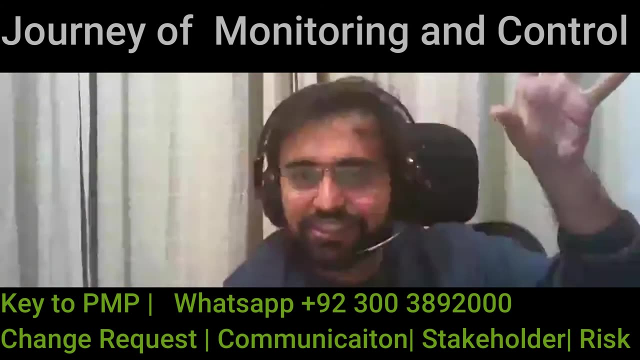 dispute resolution there and if it is not required, then close the project. so seven important things are being done. the first and most important is we are measuring the performance, checking the variances. second thing, mining the do the change request, all those integrated change control procedure. then we are verifying deliverable, the deliverable journey. we are checking the risk. 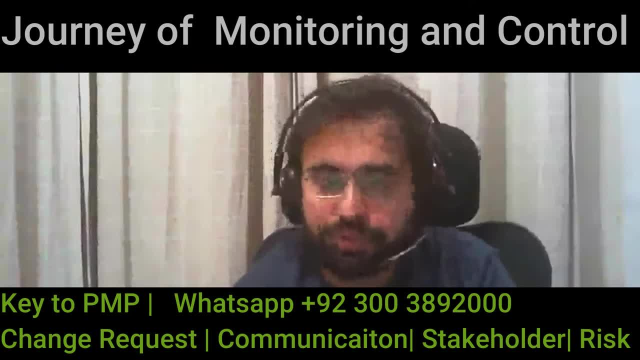 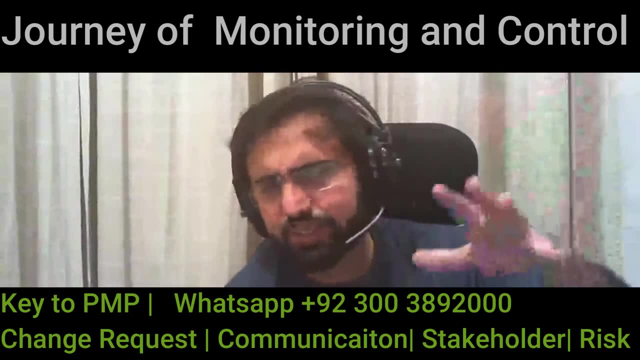 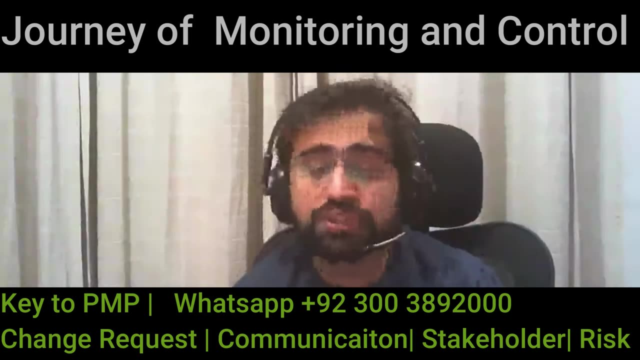 issues, writing the lesson and closing the procurement. and, most importantly, i would agree that here, like change request is also coming from execution, even initiation, identify stakeholder, even planning, from collect requirement. so change request is the biggest area. you are communicating the needs of stakeholders. of course, you are controlling. 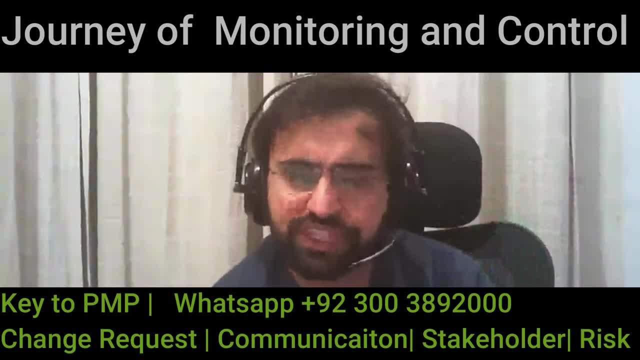 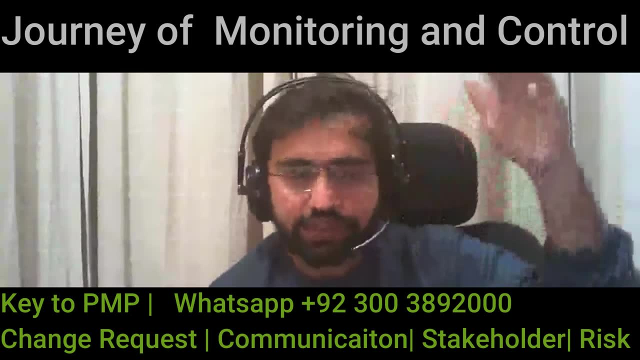 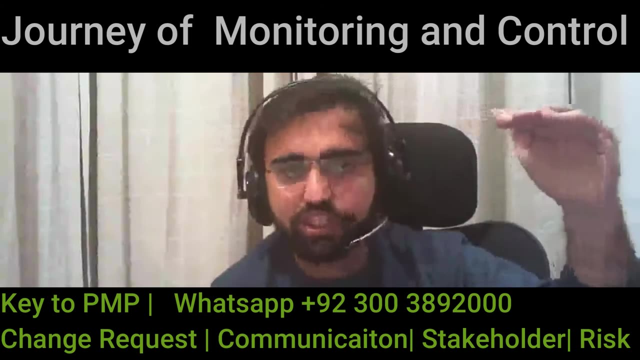 the resource and closing the resource. you are giving forecast of schedule accepting deliverable. so some flow. you need to remember the first flow flow of deliverable journey. it comes deliverable to control quality, then it goes to validate scope, then closing. then you need to see the journey of performance data journey. all the data comes in from validated.